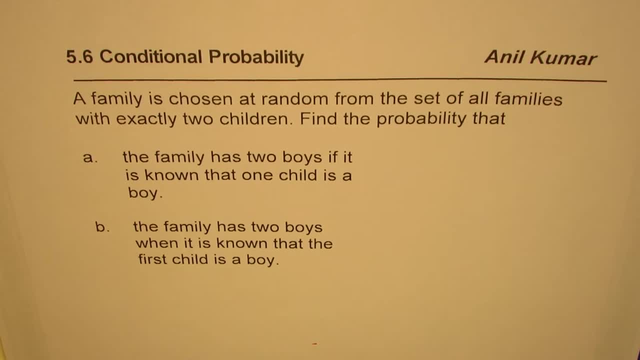 I'm Anil Kumar and in this video we will see how to find probability when few conditions are given to us. The question here is: a family is chosen at random from the set of all families with exactly two children. Find the probability that the family has two boys if it is known that one child is a 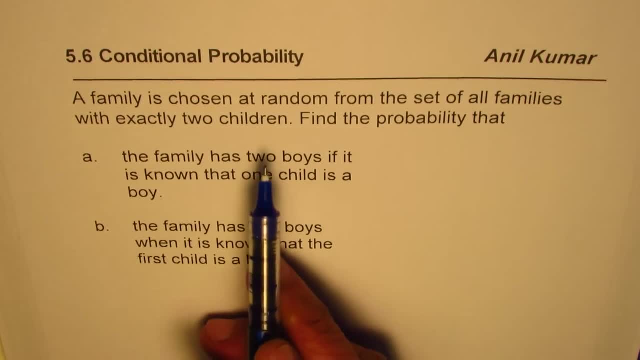 boy. Another question from the same scenario is: find the probability that the family has two boys when it is known that the first child is a boy. So we have two very related questions and in these questions we need to find the probability that the family has two boys, but we have different pre. 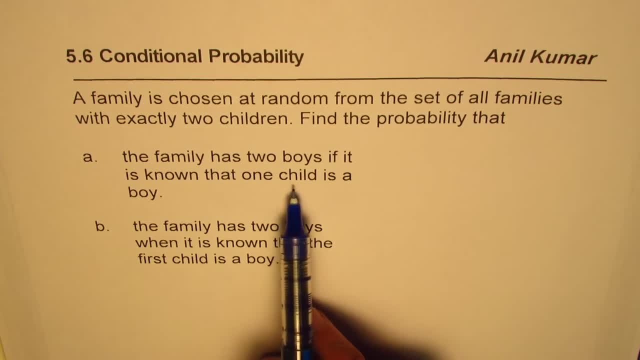 existing conditions. In the first one we are saying one of the small children is a boy, and the second one we are saying the first child is the boy, Right? so that makes a huge difference. Let us see how. So let's begin with making a tree diagram. 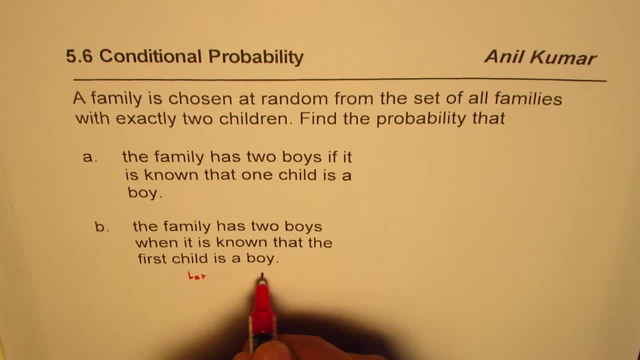 and lets say this is the first child and then this is the second child. Now the probability of having a boy or a girl is 50-50.. Correct, So we could write here: for the first child, boy or a girl, is 60 or 50.. This will be- this is 50 people, and we call the same thing as having a boy or a girl- is sarà 50-50, Then the probability for having a baby is 50-50.. If we write 50-50 across all of them in the graph: 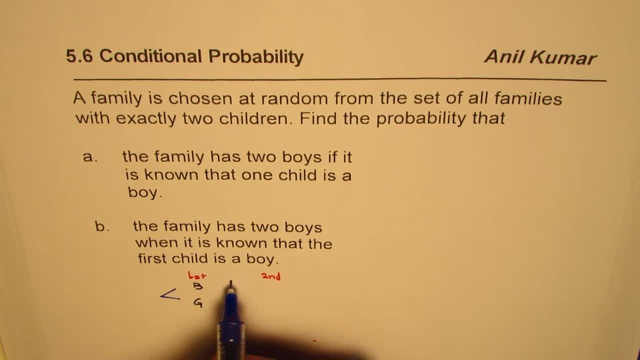 it okay, and now for the second also, it is 50, 50 great. so so we can write here: if first is the boy, the second one could be boy or a girl. if first of the girl, then also second one could be boy or a girl. now that gives us couple of 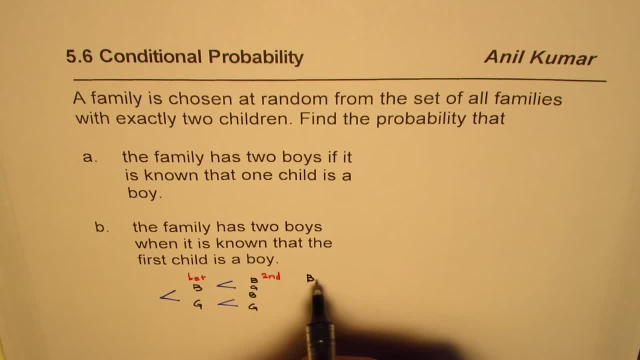 combinations. one is: we have a boy and a boy, then we have boy and a girl, then we have girl and a boy and then two girls, right? so this is the first child. that's the second child. now let's define our events. event is two boys, right, so we're. 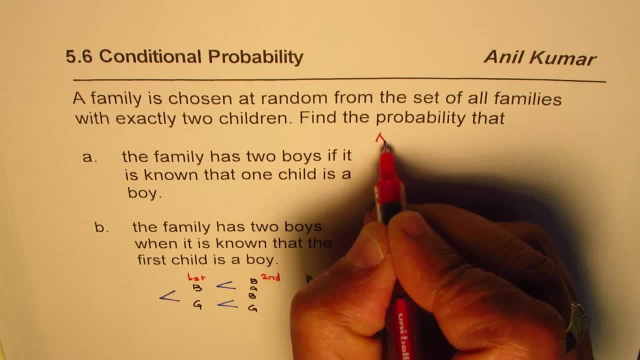 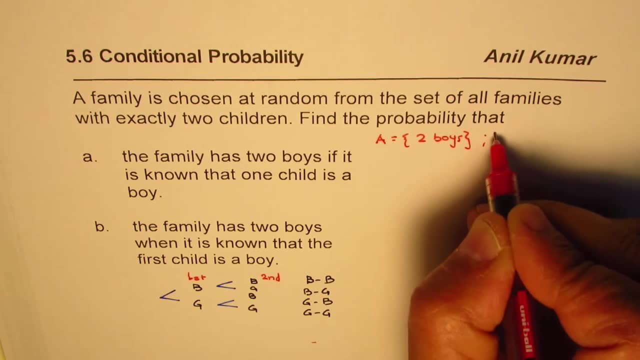 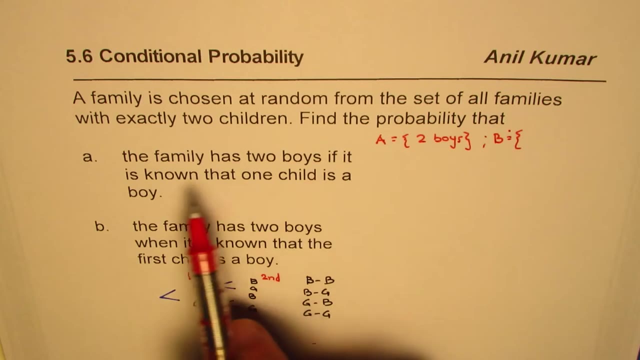 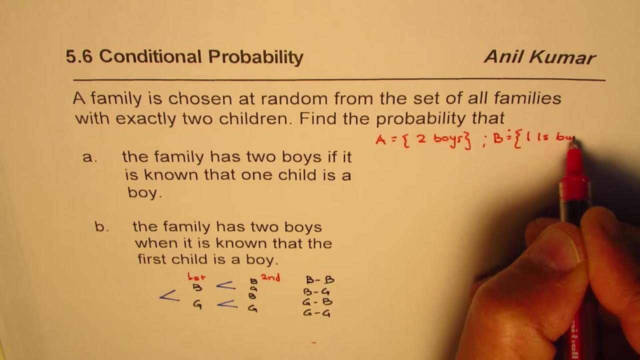 defining events here we'll say: event a is two boys, and even be in this cases, if it is known that one child is a boy, so one is boy, one is boy. right, it could be first or second, that's, that's what it means. any one of the two could be a boy. 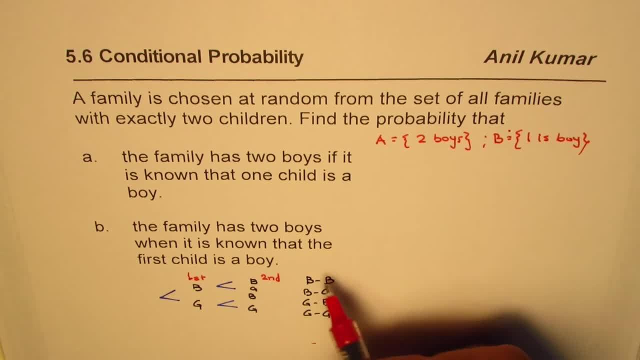 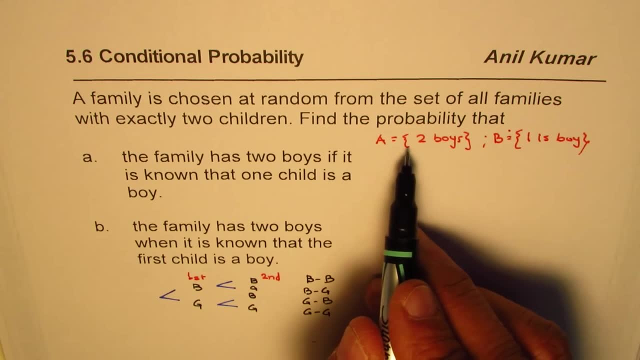 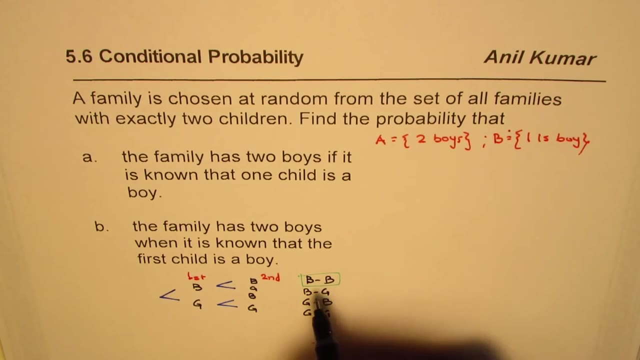 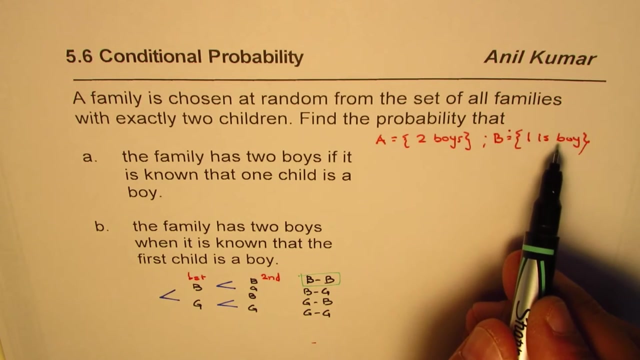 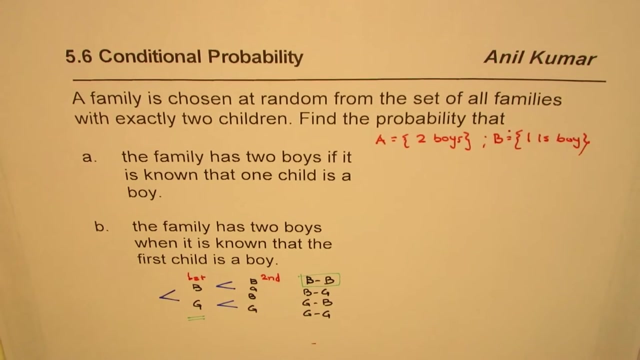 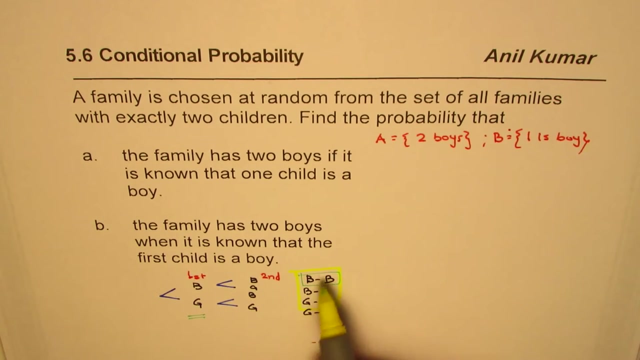 right. so that is what it is now from here. what is the probability of of a boy, right, two boys. so for two boys, the probability, is This correct And what is the probability of having one boy in the first? First one is one boy. That is, we can say these three right, These three In these three out of 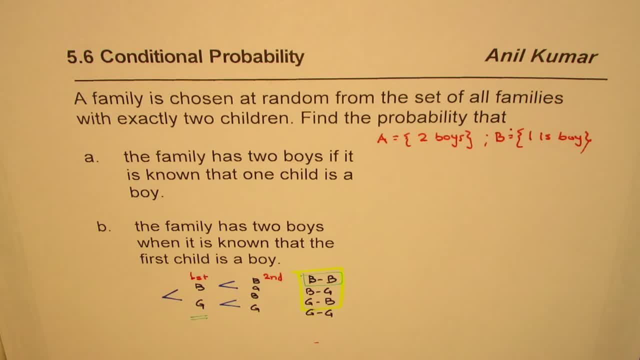 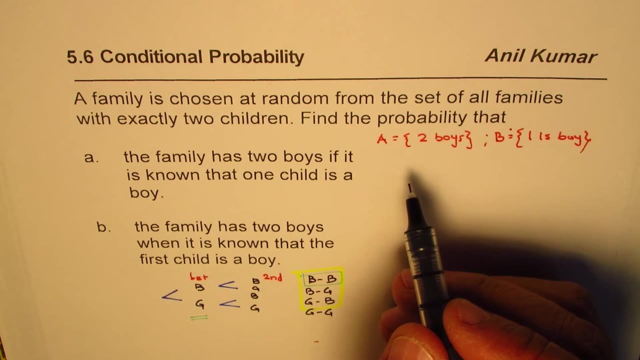 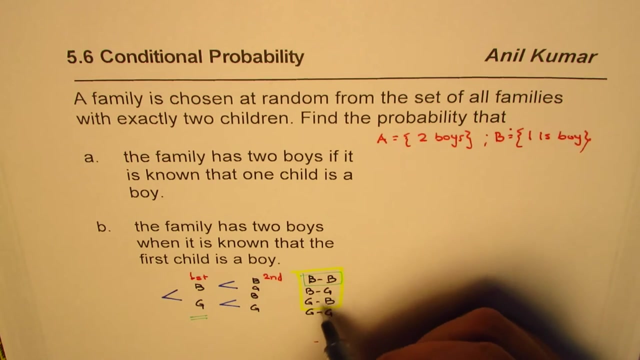 four, we find that we have at least one boy right. It could be either the first one or the second one right, So it is one of these two right. So now let's write down these probabilities also, So the probability of having one of the boys out of the four that 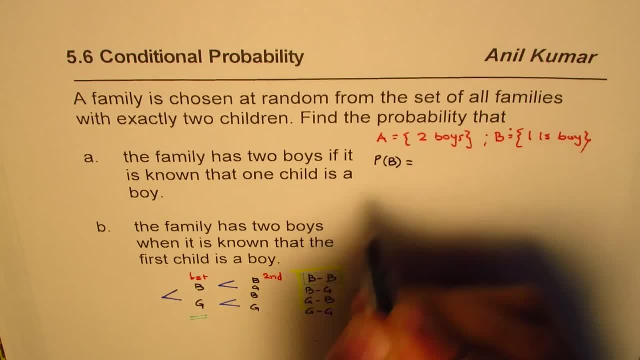 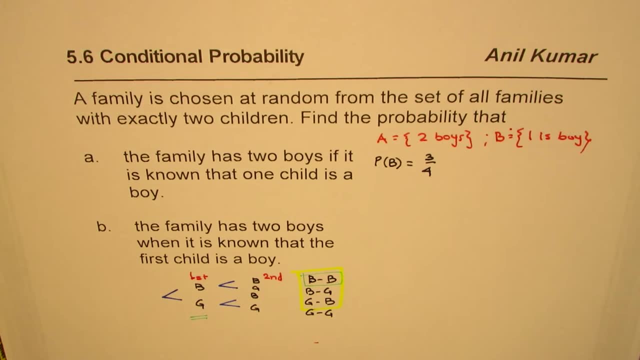 is probability for the event B to happen? Is three out of four right? And what is the probability of their intersection to happen, That is to say, when the one of them is a boy, both are boys. So we see there is only 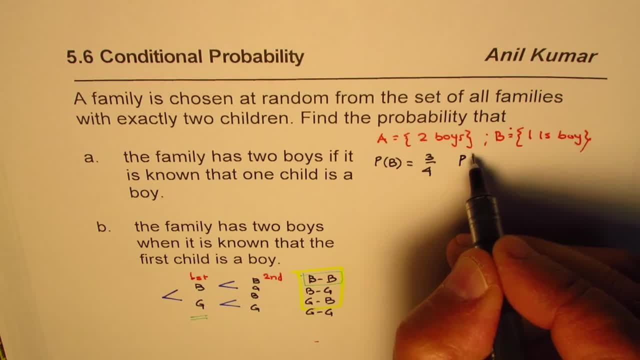 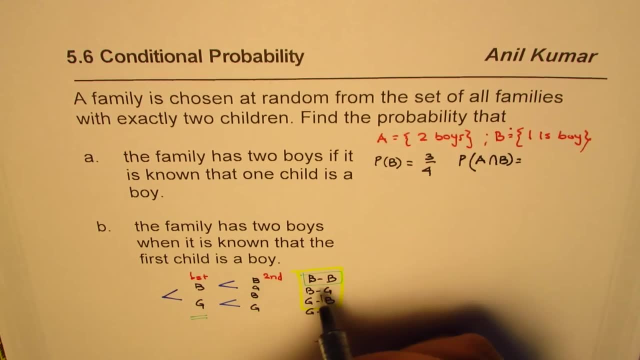 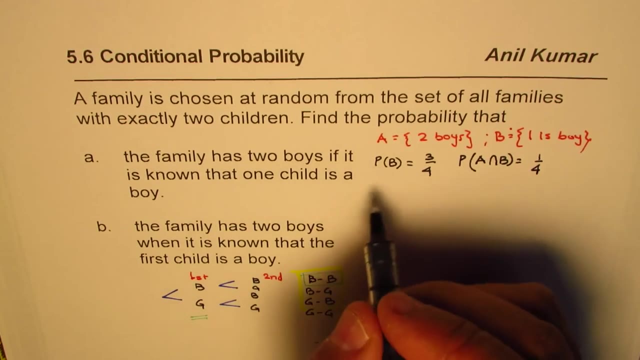 one choice right. So probability of both A and B to happen So and B to happen is one out of four. right Now, what we need to find is to find the probability when A happens, which is two boys when it. 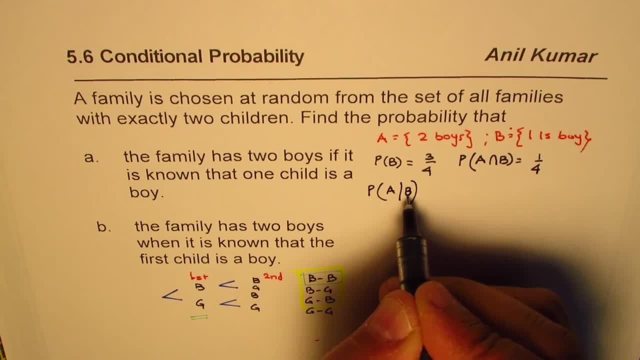 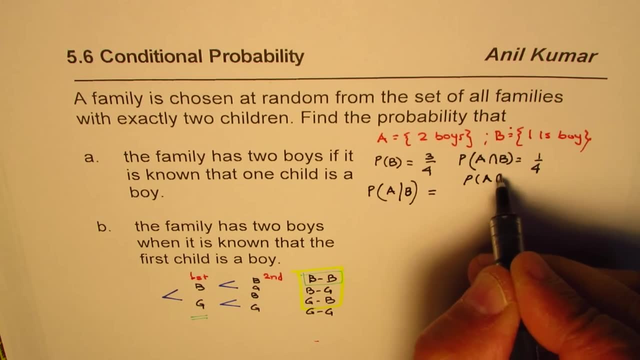 is already given to us that P has occurred, right? So B is hundred percent. That's what it means, right? For that, the formula is probability of A intersection B divided by probability of B. So in our case, probability of A intersection B is one over four. This 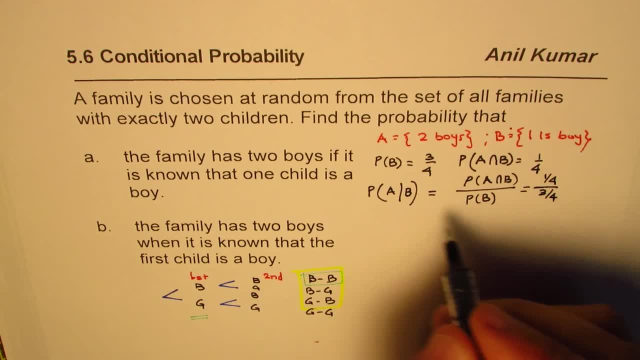 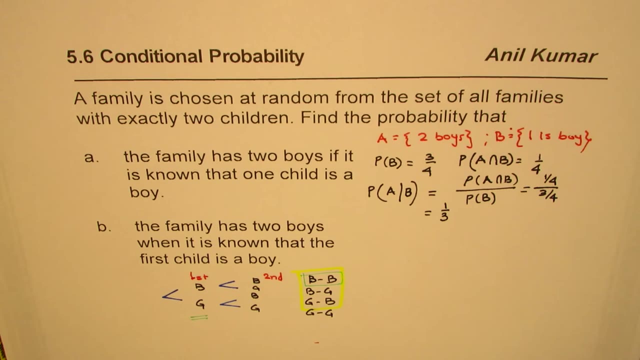 divided by 3 over 4, right, And that gives us a value which is 4 over 4. cancels, we get 1 over 3.. So the probability of a family having two boys, if it is known that one child is a boy, is 1 over 3.. 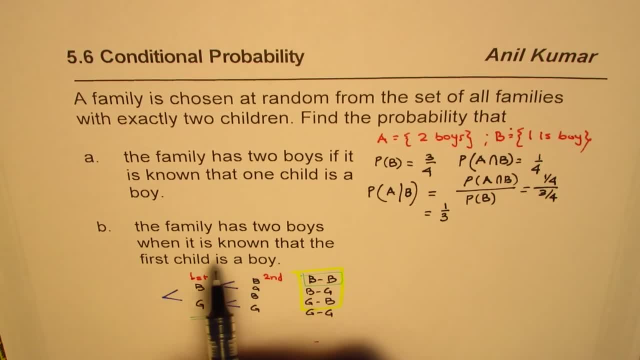 You get the point right Now as to the second. the second condition is the family has two boys when it is known that the first child is a boy, right? So first child is a boy. that means we have two options. 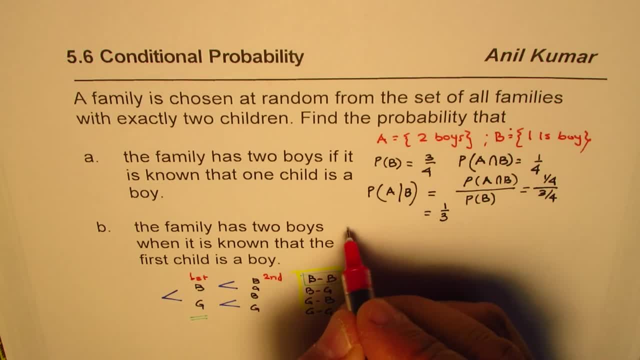 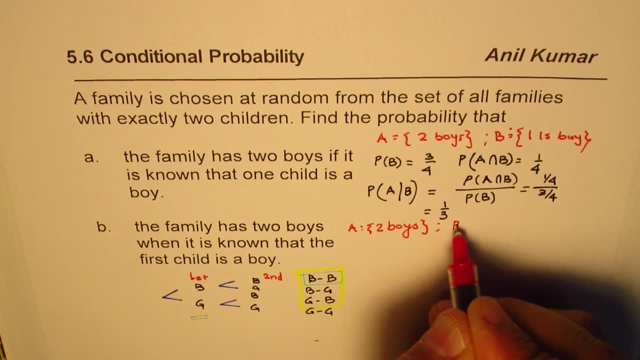 So in this case the event B. so event B- A is same. for us. We say: event A is two boys And event B is first boy. Okay, So in this particular case the probability when event A happens and B has already occurred. 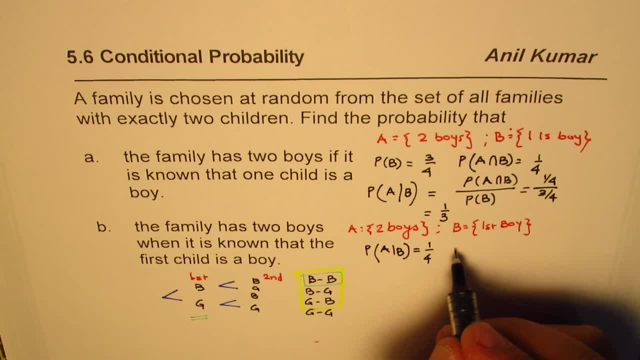 is 1 out of 4, as it was last time. However, the probability for event B to happen- that means first one to be a boy- is 2.. There are only these two right. Where first one is the boy, is 2 out of 4.. 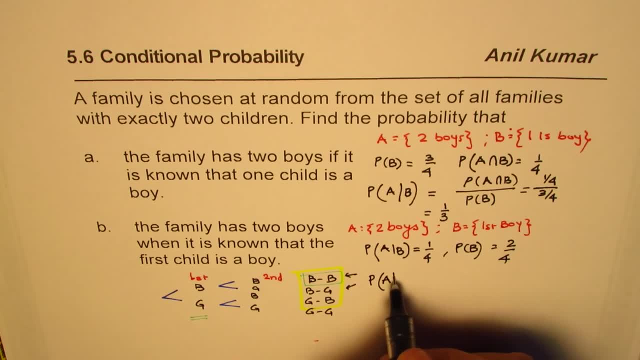 And therefore the probability of two boys when the first one is B boy is written as probability of A intersection B. I mean this was intersection N, right, Okay, Divided by probability of B, which is 1 over 4, divided by 2 over 4.. 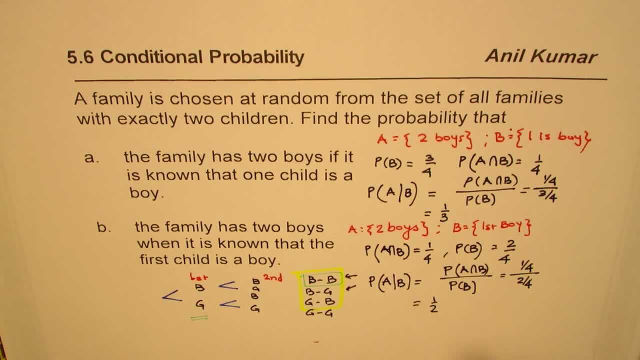 And that gives us the answer: 1 over 2 is 50%. Do you see that? So it is 0.5 over 50%. So in probability questions the answers may differ If pre-existing conditions are different, as we saw in this example.